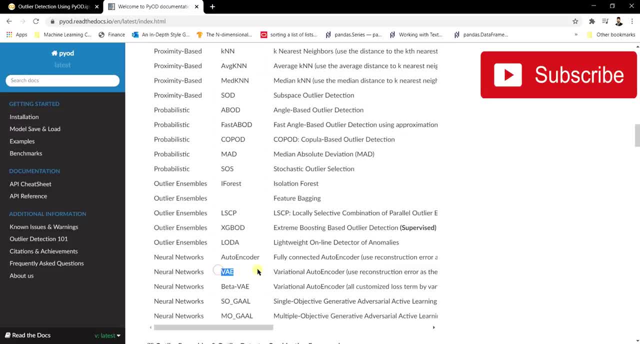 library, which is encoder, variational encoders, beta variational encoders. So such kind of models even have been included into this library. So that's because of this reason it's an effective way of detecting the outliers in a data with using various kind of outlier. 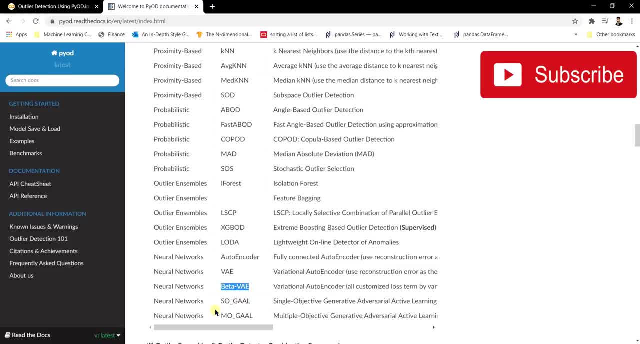 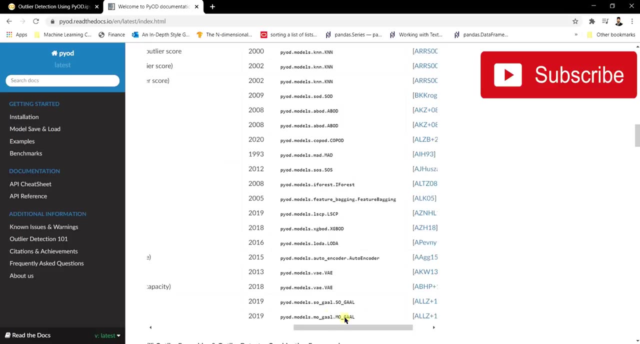 models- outlier detection models. So recently it didn't work. Recently they have added the latest outlier detection models, which are single objective generative addressable learning models, And even this multiple object generative addressable active learning models, So which is generally been introduced in 2019.. So these are the 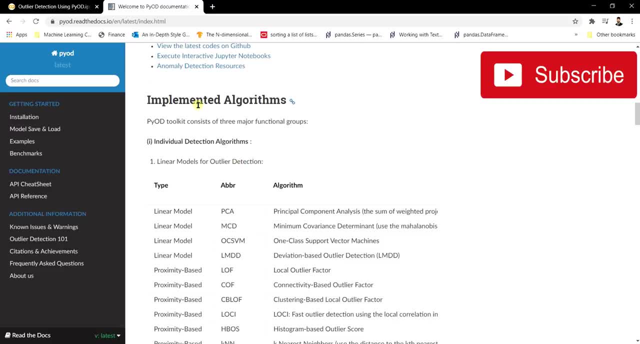 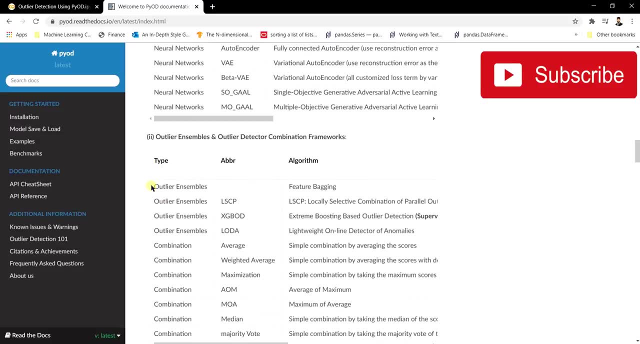 algorithms which are being introduced into this PIOD And even further. if you go scroll down below, you'll get to know that there are also outlier assembled models available in here. So I'm sorry, I don't want to get too into the details of this, But you can use the. 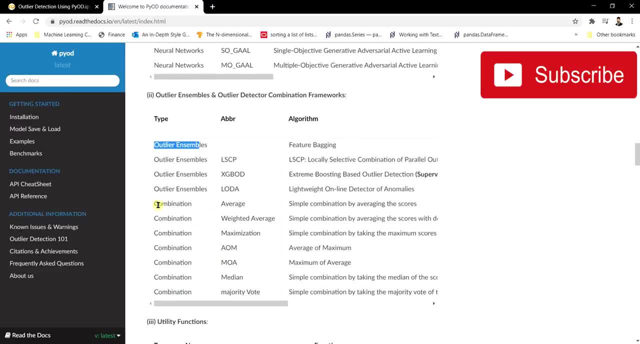 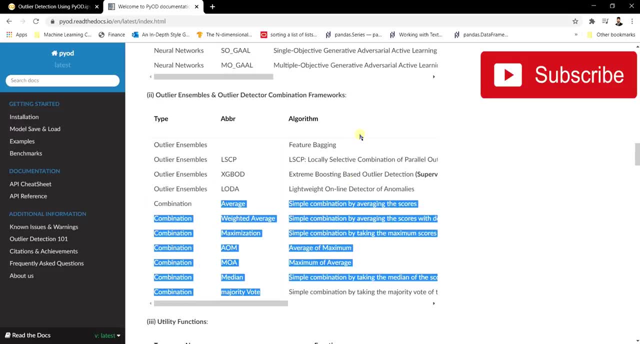 combinations of these models all over these models, And you can also prepare your own custom models by using these kind of functions that are available over here in this library. So this is what a helpful library looks like, PIOD, And it can be very, very helpful in. 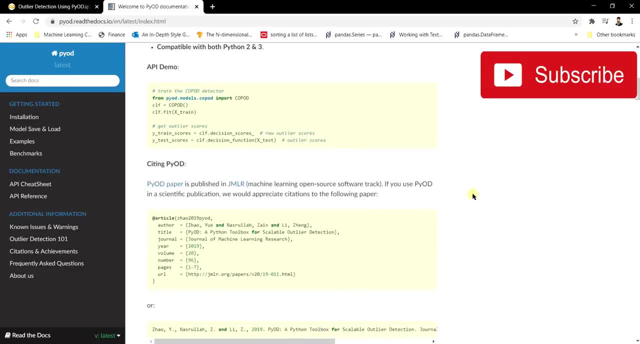 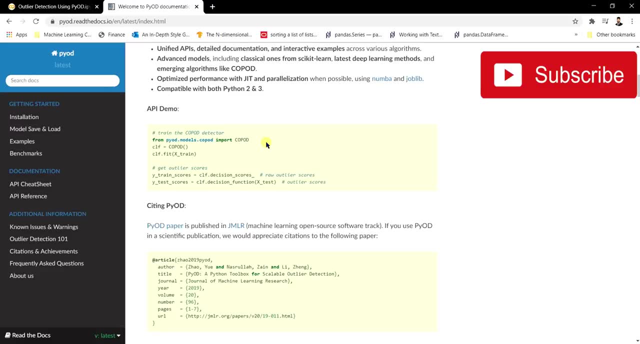 our outlier detection. So let's see and understand, like how to be helpful. So let's just jump back to the collage and understand a few of the algorithms which are generally being used in detecting the outliers and let's walk through a simple implementation of. 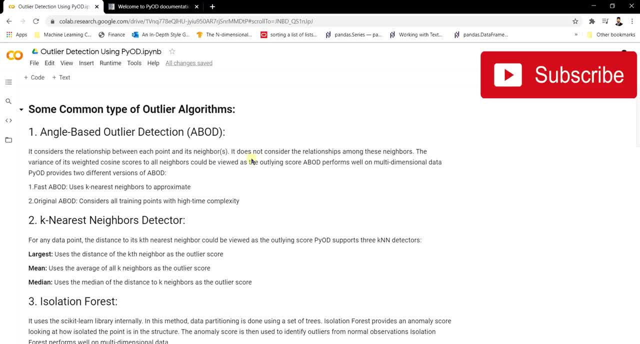 pi hodi. so let's start. so here i have listed some common types of algorithms which are generally being used in productions. so let's walk through these algorithms briefly. so let's start with the first one, which is angle based outer direction model. so this angle based outer direction model. 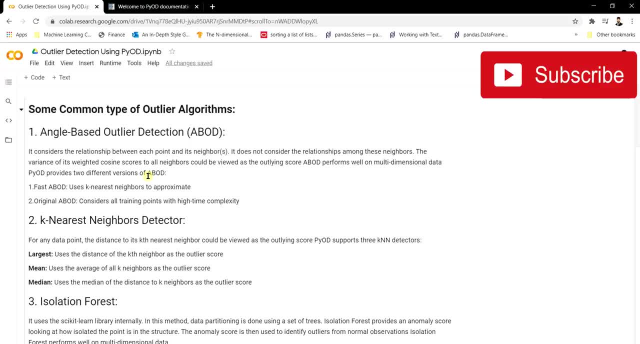 consider the relationship between between each points and its neighbor. it measures the cosine scores between each of its points and its neighbor and gives a variation of its weighted cosine score. it is well perform. it is it generally performs well on multi-dimensional data and there are two ways of doing angle based auto detection, which is fast, abod, and and and another one version is: 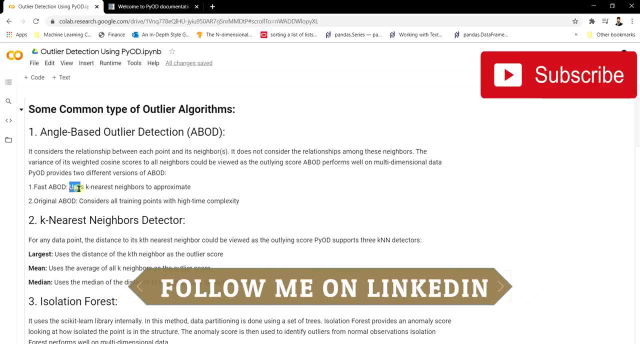 original abod. so fast abod uses k nearest neighbor to to the approximate version, which generally gives an approximate version of this abod. and the original abod consider all kind of complicities, which generally uses cosines, scores and everything. so these are the two variations in this angle. 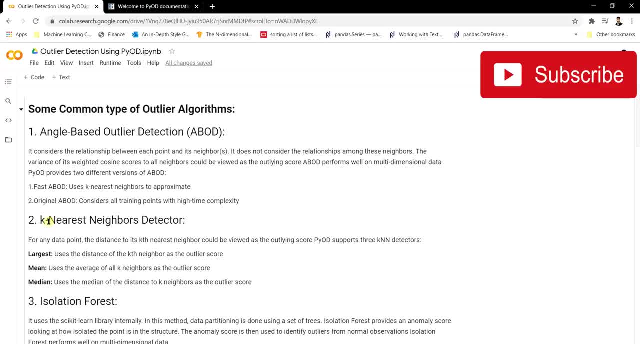 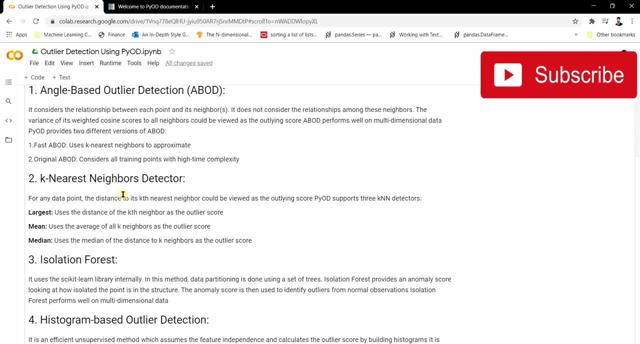 angle based outline direction model. and the second one is k nearest neighbor director, so as the name signifies that it uses the k nearest model, which is which generally measures the distance between each and every points by using equally distance, and, and it and it gives the outlier based on this distance. so if a distance 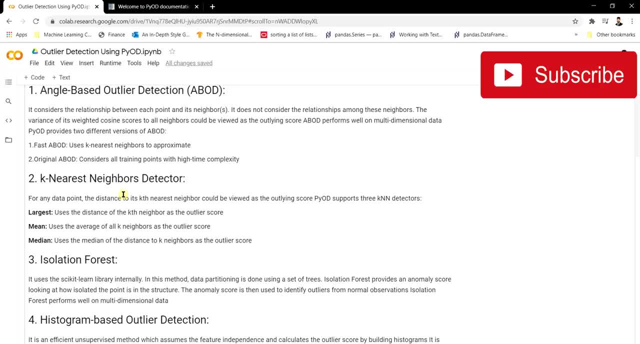 is larger than the other points, then that particular point which has larger distance, will be classified as as an outlier. so this is what uh, k-nearest model, k-nearest model director does, and it has also has three variations: which is large, mean and median. so largest one is uses the. 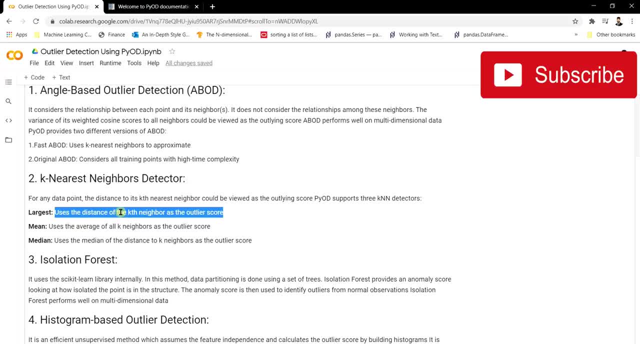 distance of the k nearest as the outlier. so it uses the largest distance of the gay nearest player as the outlier. use the average of all the k-nearest brothers and neighbors as an outlier school. so it uses all the distance measured and takes the average of it and consider as an. 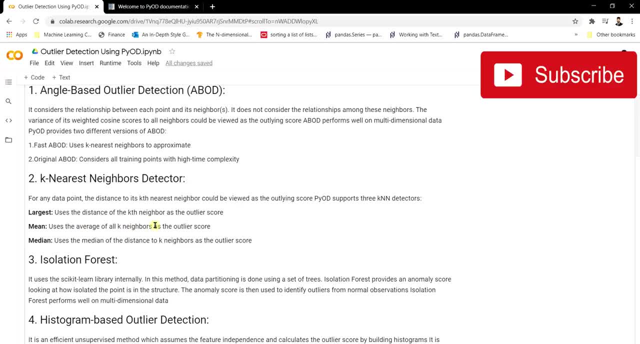 class. so if the distance is greater than the mean score of all the uh k-nearest distance, so it classifies those uh points as an outlier and median score uses the uses the median of the distance of the k nearest neighbor as an outlier. so this is what a brief. 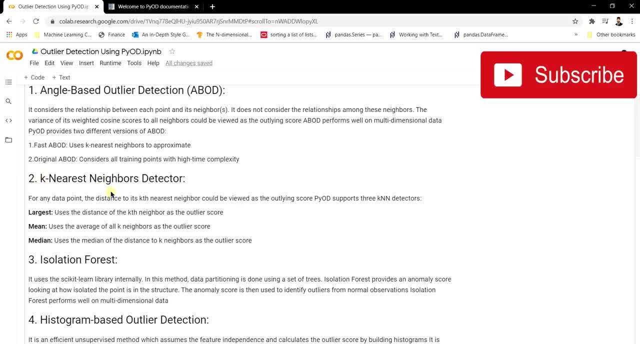 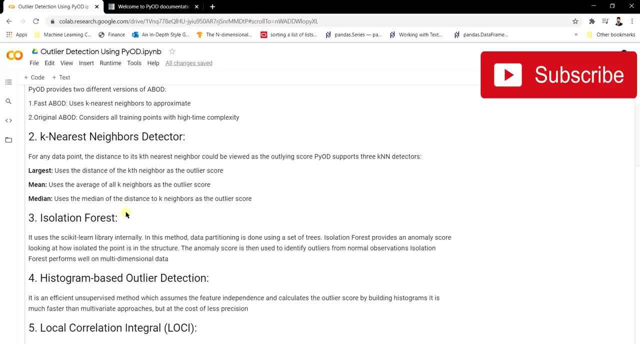 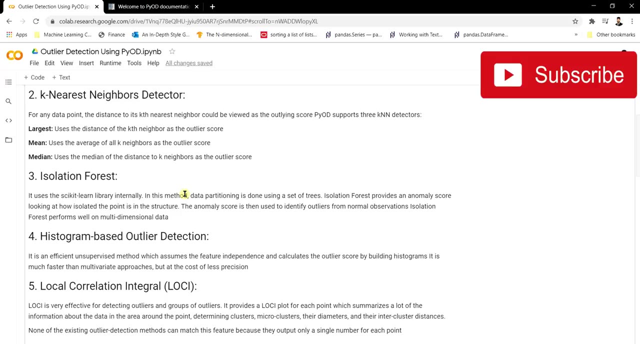 general general induction to the k nearest detector model is. so there comes an isolation of forest as well. so basically, what it does is it creates, it divides the data into different trees by using different trees and then the, and it measures the data points which are lying outside these trees. 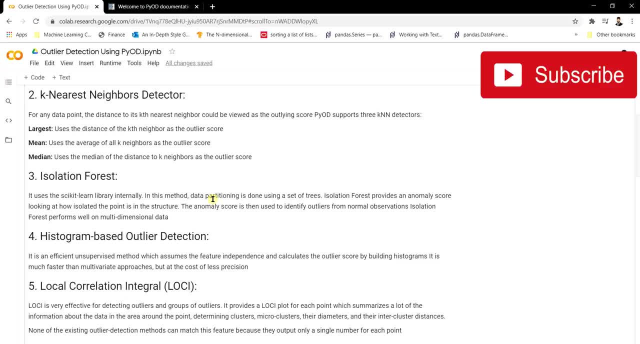 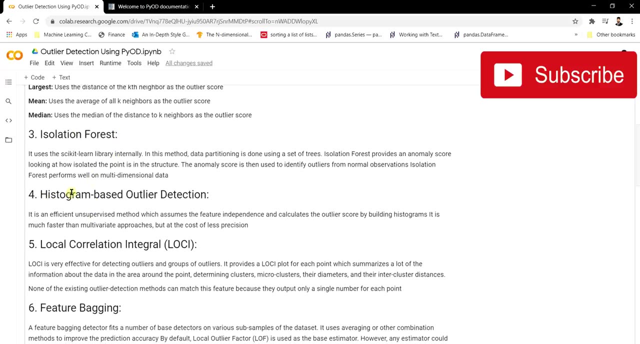 so it considered that as as an isolated data point and generally called as out there. so this perfectly works better in multi-dimensional data. so this is all about this isolation forest. and there's one more algorithm which is called histogram based outlet action, so it generally uses histograms to build upon the outlay. so if that particular data points are above histograms, 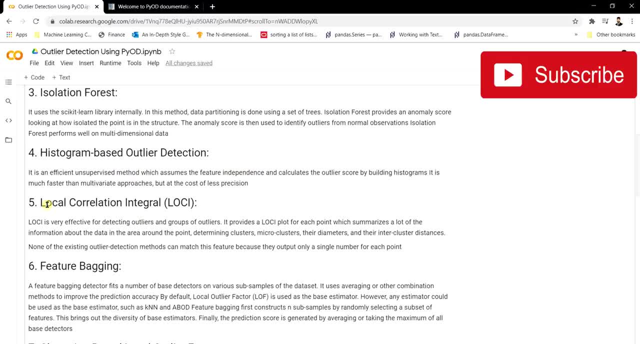 so they're generally considered as an outlier. and there's again a very special kind of outlier action model which is local correlation integral model, which generally takes on depth data points and cluster them into and many clusters and micro clusters and with their particular time diameter specified, and then it measures the 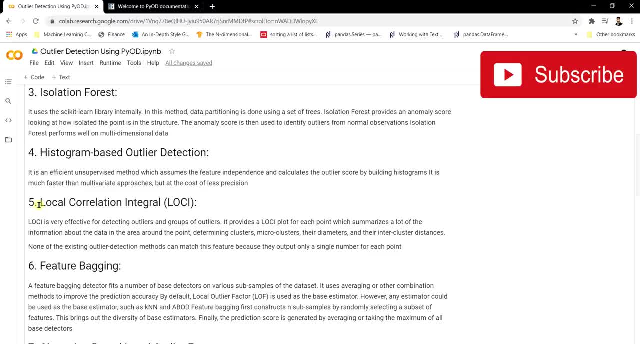 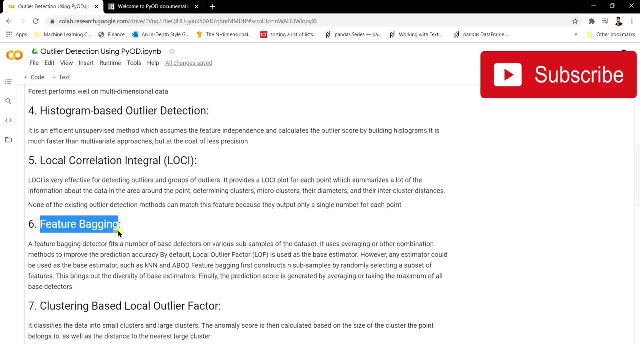 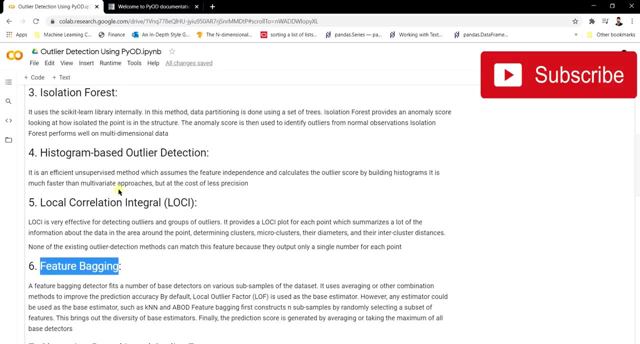 inter cluster distances and specifically because of the inter cluster distances it classify as an outliers point. and we have feature packing as well, which which takes the combination of these uh outliers, kind of reduction models, all the kinds of reduction models, so you can take any kind of like local correlation model and histogram based. 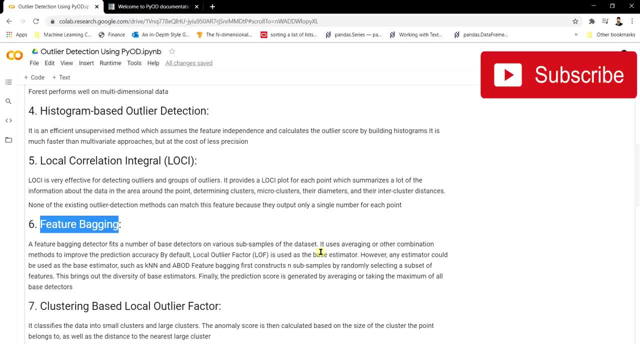 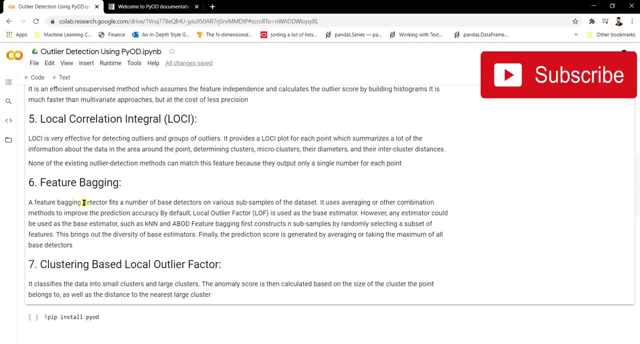 or architecture models and combine their outputs and present it the outlier model. so this is what a feature backing model does internally. you can even change it according to the use case, and the last one which I would like to discuss over here is clustering based local outlier. so what it does is it? it classifies the data into small clusters and large clusters, and the 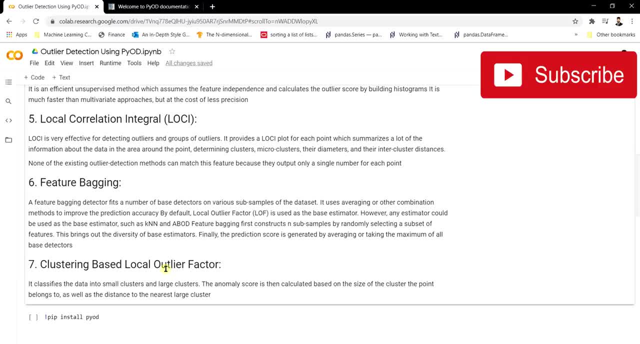 anomalies course is then calculated based on the size of the cluster the point belongs to, as well as to the distance of the nearest class cluster. so what it does is it: it takes the, it forms the clusters and it measures the distance between those small and large clusters and according. 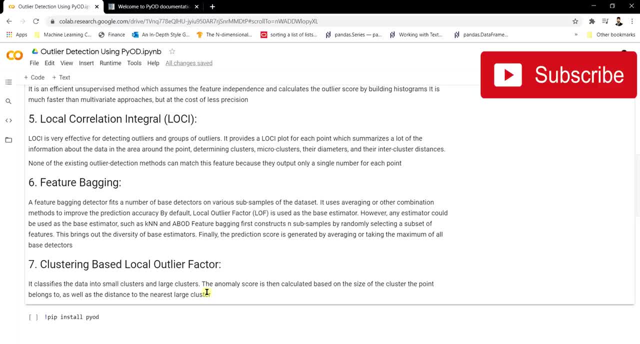 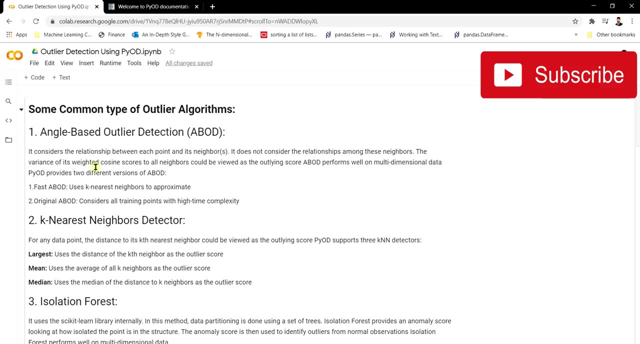 to that it, it assigns the score uh to the model and based on the distance, and then it and it assigns the cluster as an anomaly. so this is what a general overview of these kind of uh models which are generally used in production level to detect the outliers. so now let's just walk through. 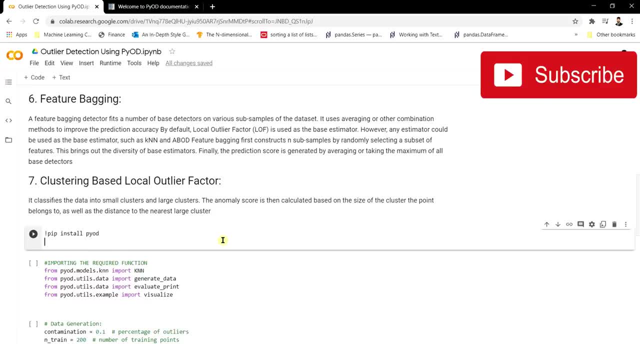 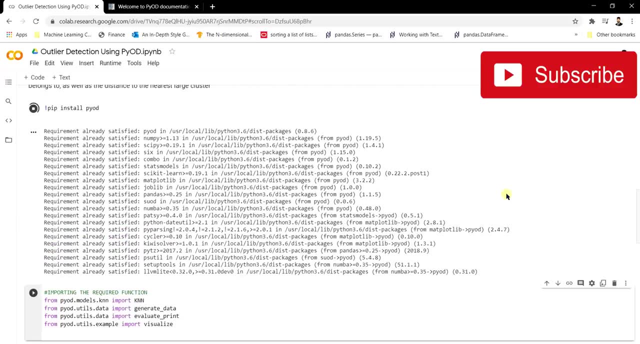 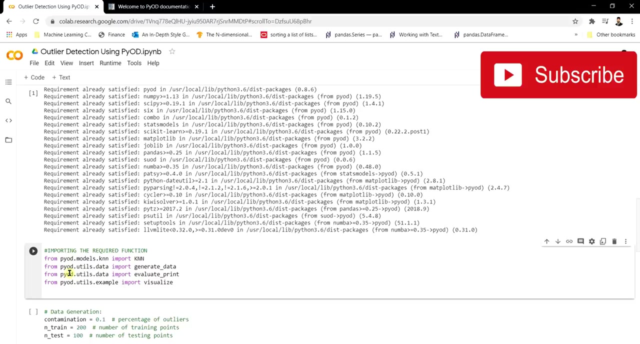 the simpler implementation of this piod. so first we need to pre-install the piod library, as usual. so let's run this cell. so as I have already installed this by already on my this uh collab cluster, so it's it's already requirement satisfied. now we'll we'll import a few of the functions which are required. so let's. 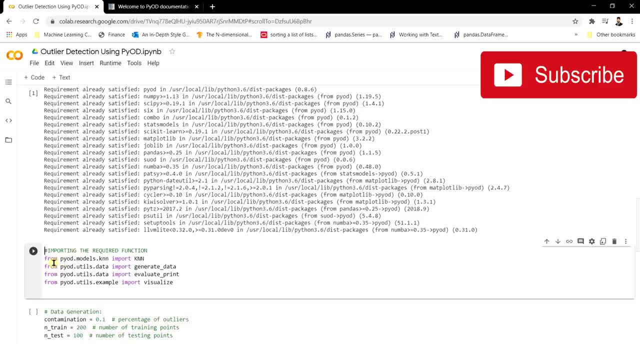 walk through these functions first, then we'll import it. so from pi model, from piod dot models, we are importing canal cluster model. so right now, for the demonstration purpose, I am using k nearest neighbor detection model. so that's what I'm importing from piod and I'm using 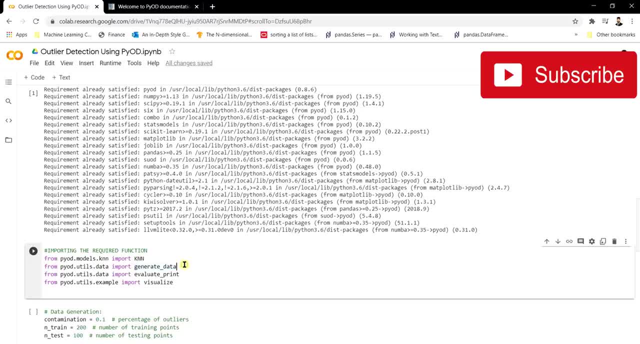 uh piod data generator function. we generate a synthetic data for the outliers, so we are importing it from the piody, which provides a simple function to generate data, and then we are also importing evaluate print, which will give the accuracy like precision and recall. so this function will help us to evaluate the performance of the outlier model and we are 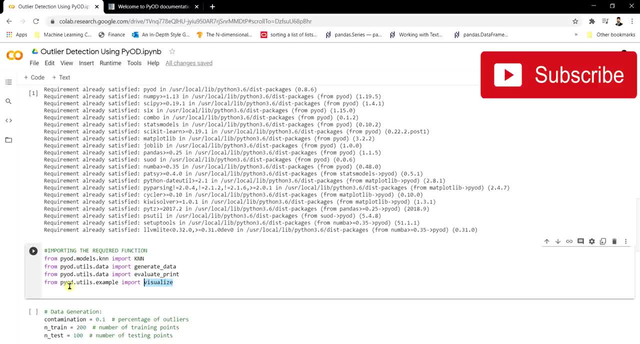 we are. we are again importing uh from the piod library visualization function, which will help us to view the different kind of uh outliers from uh, from original as well as printed mod. so, uh, let's run this, run this cell and we'll understand everything uh in just a second. so, uh, like how these functions are working. 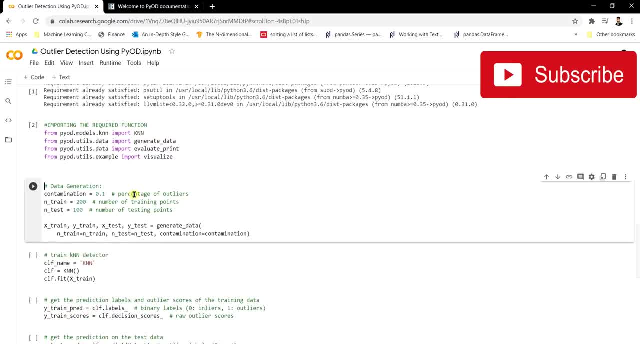 and how it will be helpful to understand this piode library. so our first implementation would be to generate the data. so for generating data, I have taken uh 200 train samples and 100 test with 0.1 outliers. so that means 10% of the outliers will be present in that data. so for 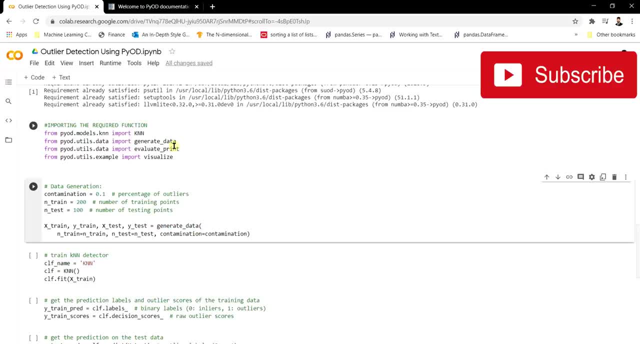 generating data. we are using generate underscore data function, which I have imported from this PIOD and specifying is all the parameters in it and will generate the data as X train, Y train, X test and Y test. so this will generate this data- X test and Y test- and then we're. 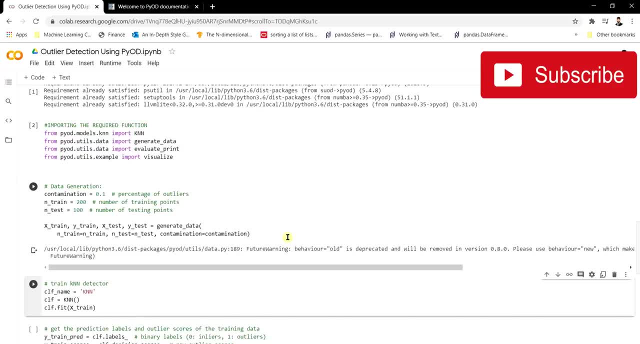 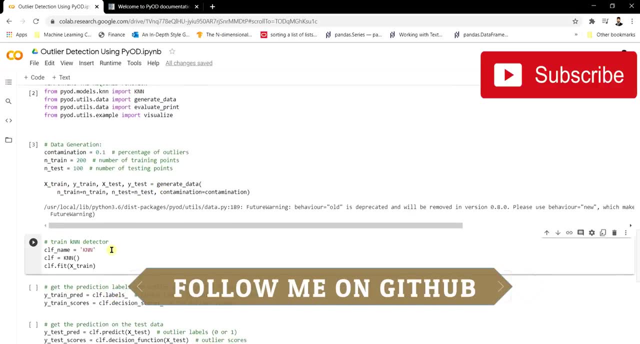 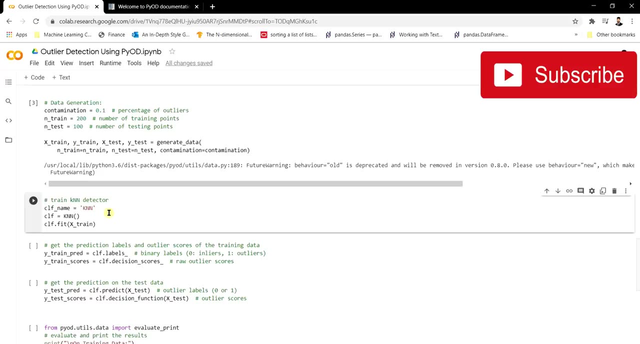 gonna be running this cell, so let's run it. so as the code ran and we got all this data generated and so now we're going to be initializing our algorithm, which we're going to be using it. so we are using over here is KNN, so let us run this and fit on this X train. so remember, we are not. 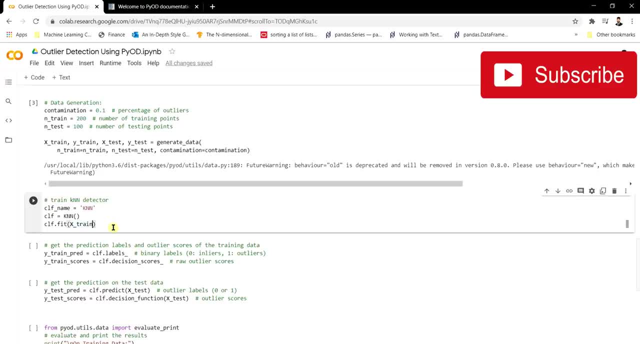 fitting it on the X train and Y train as we generally used using x-clanning and xstrain and xstrain library. here we are only fitting it on extend data and we are using y train to consider the consider the performance of the model. so let us run this. so the 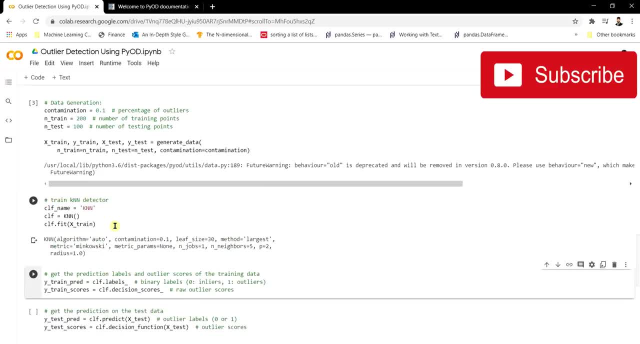 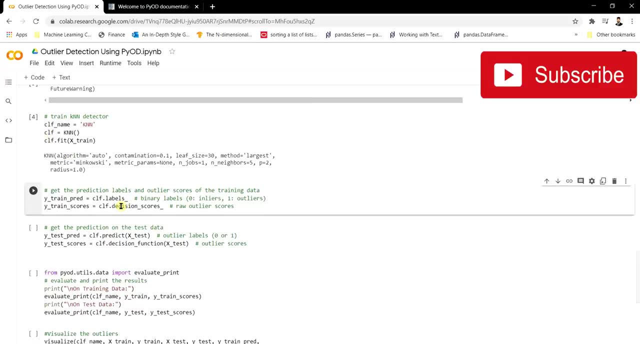 model has been fitted to the train data and now we're gonna be using the different kind of function available here in this classifier. so classify has this method called label, which generally prints the train labels like when, when this model has been trained using this X train. so, whatever the 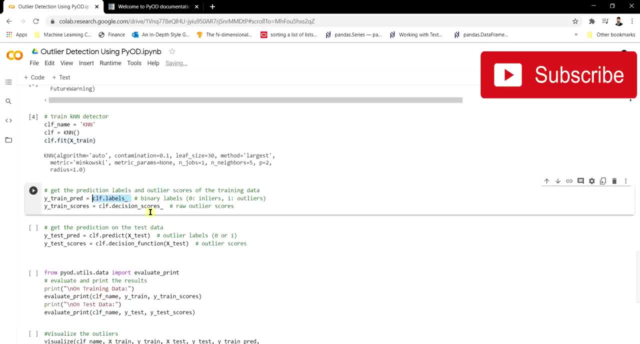 labels it has printed at, whether it is an outlier or it is not. so if it has printed at zero, so it is called inliers, and if it is printed as one, then it is, it is called as an outlier. so this is what classifier dot label and labels. 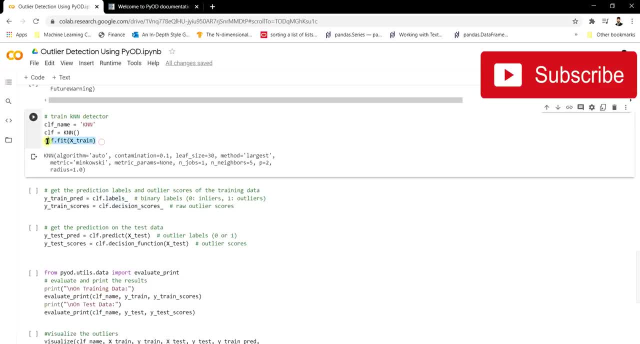 underscore method is working over here, so it is. it is working on this train data, so that's what I have stored. this: this outputs from this method to y underscore, train underscore, pred variable. and similarly we have given we have a decision score method available in classifier which generally gives the scores score of the model, so let's run. 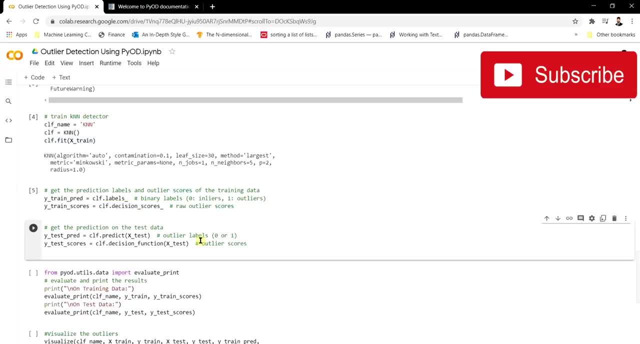 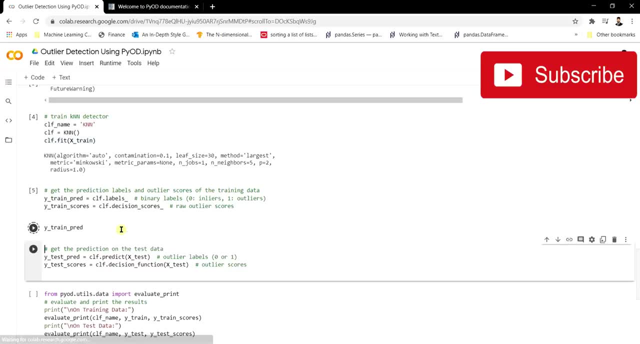 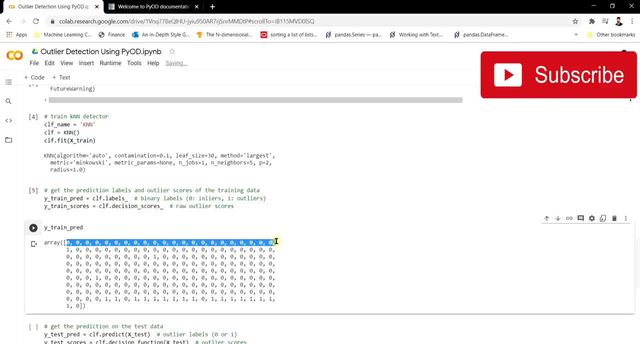 this and let us see the output. like what this y underscore, trainers, Patriot- consists of. so let's run it. as you can see, it generated a binary outputs. so these are the outputs of the model, which generally says that these are not these little points and not outliers, and in between it has one as: 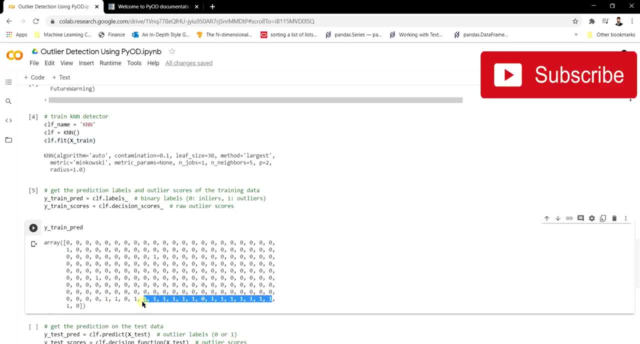 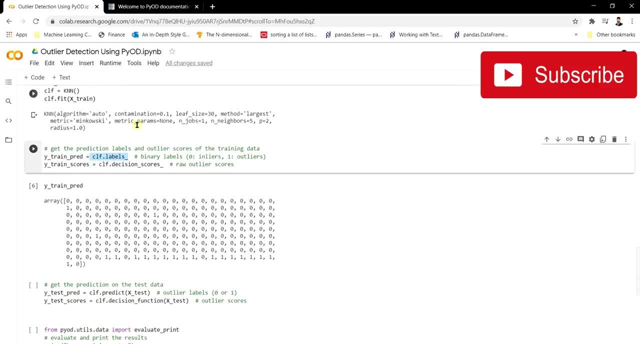 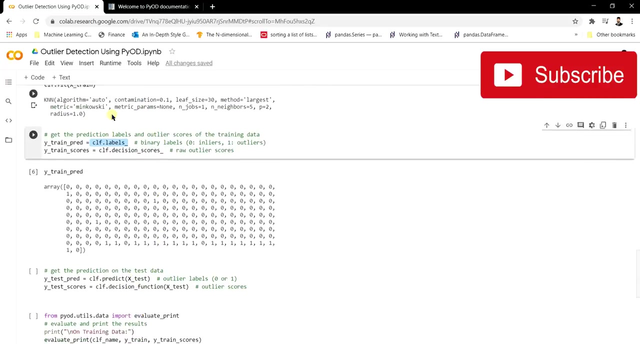 well, and the below you can see their phrases, or one as available, which is suggesting that it is an outlier. so this is what y underscore trainer scope rate has has in it, which comes from the classified out labels underscore method. so this is all about this uh train part, and now let's move to the test part. so now, after training this model, on this x train, 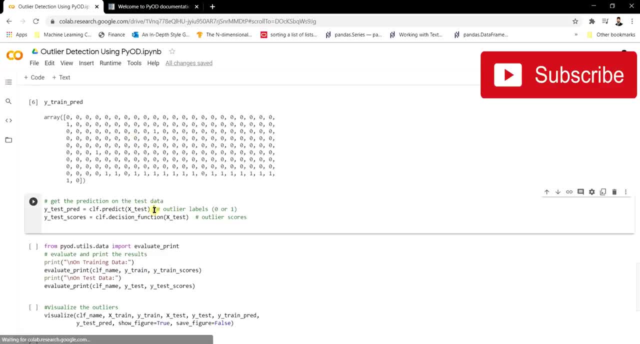 we want to get the prediction on the test data that that, whether that uh classifying that particular test data points as outlier or not. so we'll use clf dot print method and pass the test uh data into it and then it will create the labels: which is zero, zero and one. so if it is zero, that 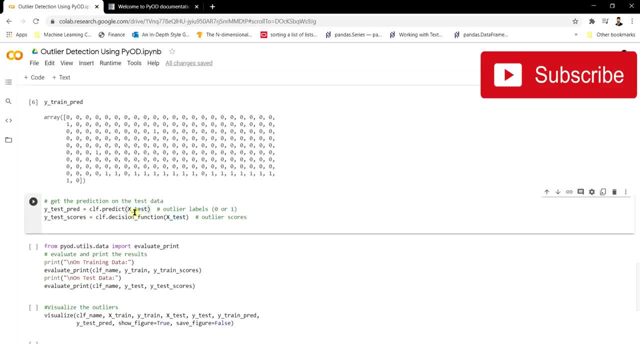 means it's not an outlier and if it is one, that it's an outlier. and similarly, we're going to be using this clfdecision underscore function on the test data, which generally means that it it predicts the scores of outliers. like what the performance of an outlier method. so generally uh gives the 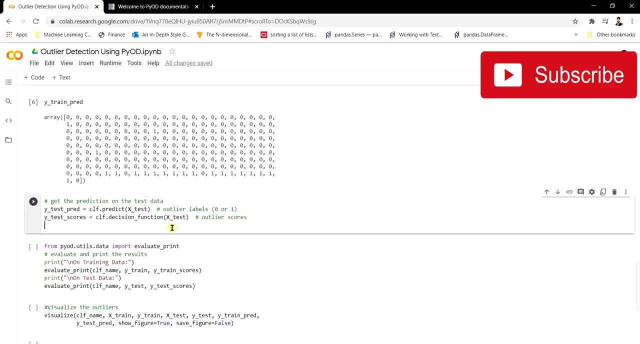 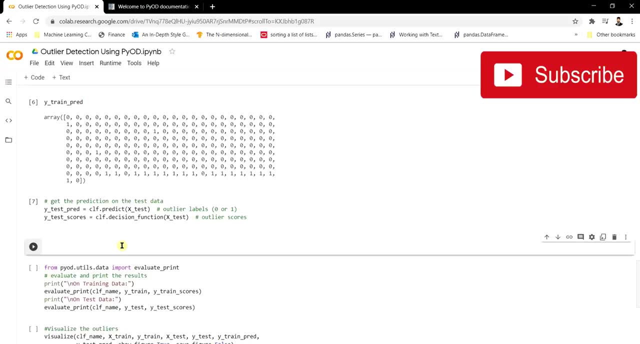 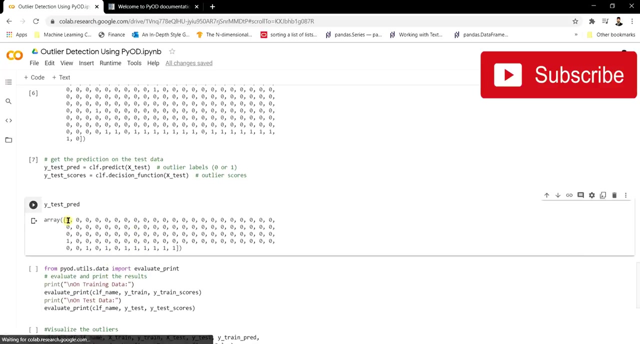 score of an outlier. so for this, we just run the cell and let's, let's see what does this looks like. so let's run it. so now we're going to be seeing the test results, which has been printed as 0 and 1. so let's run this variable so as we can see. uh, these are the uh test points. 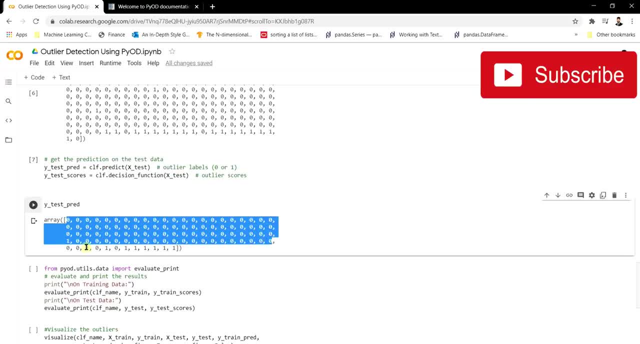 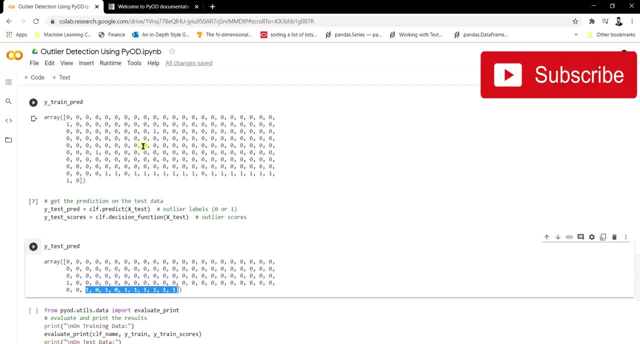 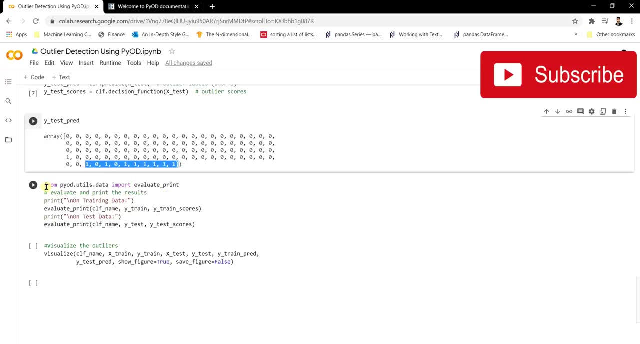 which have been printed as an uh, not an outlier, and here are the some ones which are. which model says that it? these are outliers. so this is what the k-nearest neighbor model is working, and let us take these things in a form of precision recall. so we are importing this: evaluate underscore. 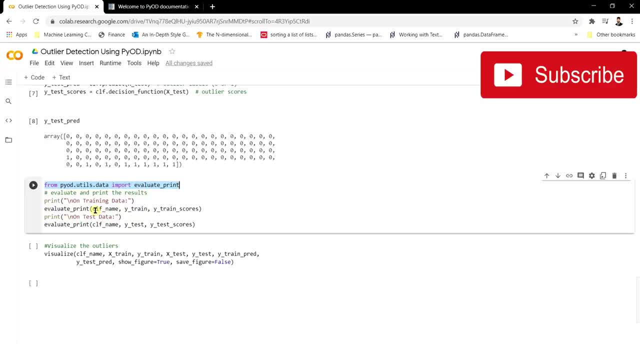 print function from this pi od and we are passing this class, classify name and y train and y train score. so we're just testing it on the train data set first, like what we have trained it on, and now we are taking the uh, so don't forget that uh. similarly, we are using some Illinois Huh communications. 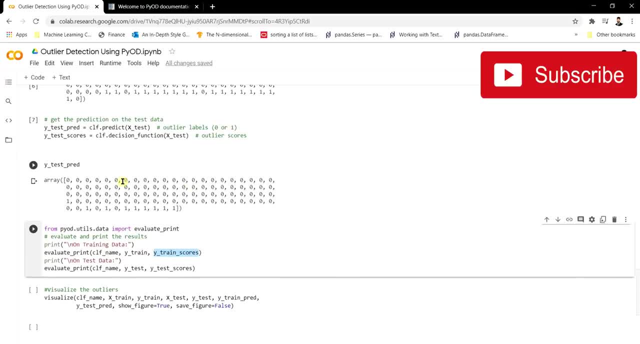 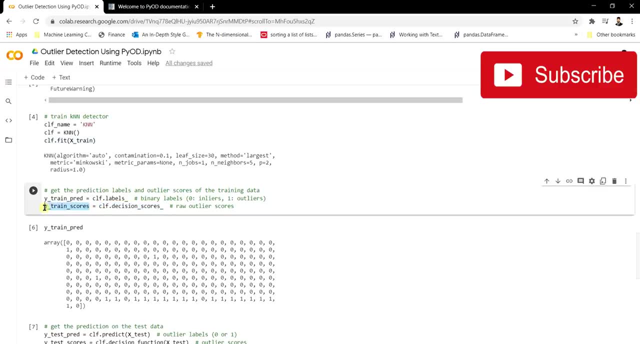 because that the same defined behavior to theそう. that is the one we are working with, but we've done uh, similarly we are doing with that test data as well. so remember: the strain y underscore trainer score scores comes from over here, from the decision score, which is available. 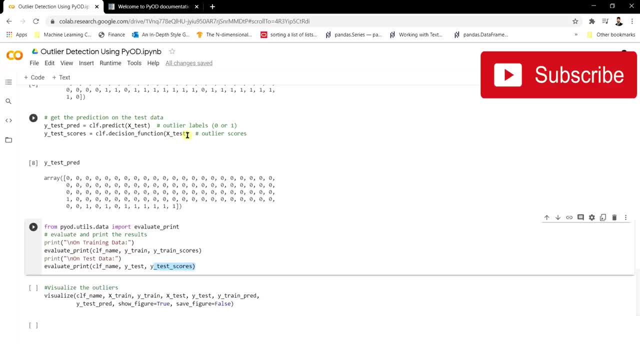 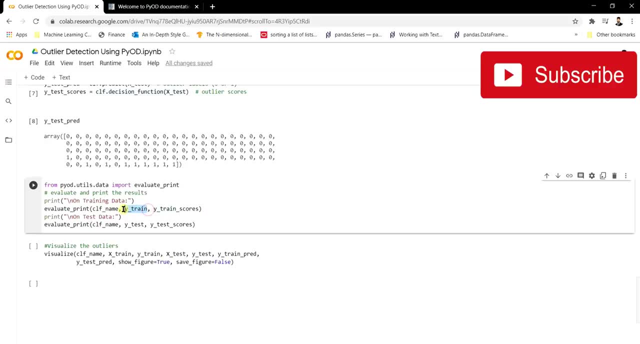 or over here in this trainer score of variable and and why it underscore test score comes from here, from this decision function. so we're going to be using this, this, these two variables, and with the asks 장이, train and y test, and you are evaluating on this train and test data respectively. so let's run this. 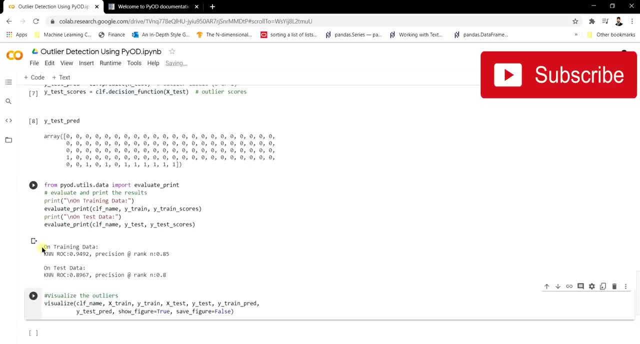 so, as you can see, on the train data, the knn roc is 94 percent- like approximately 95 percent- and precision is almost 85 percent. and our test data, uh, the knn roc is almost 90 percent and precision is 80 percent. so this is what an evaluator scoop print is working. so it is giving the performance. 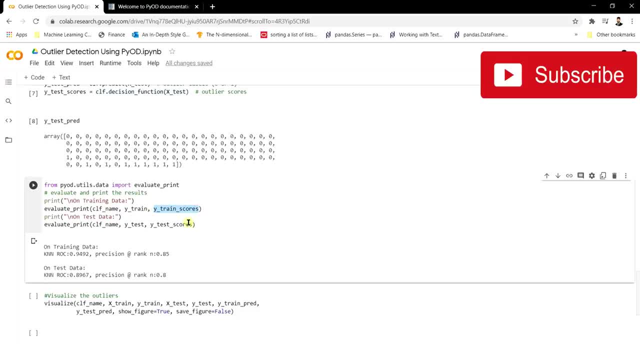 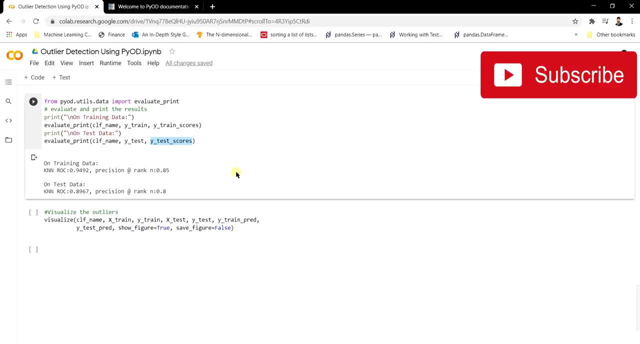 of a model by using this, the scores of the outliers which we have used by using the different methods available, available in the classify method. so in classify function and let's visualize these things, uh, to get an accurate understanding of this priority functioning. so so for visualizing the 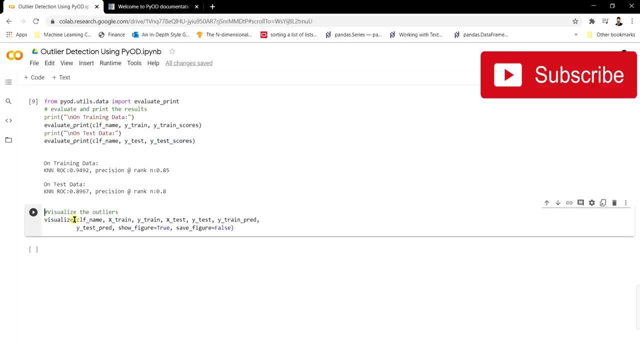 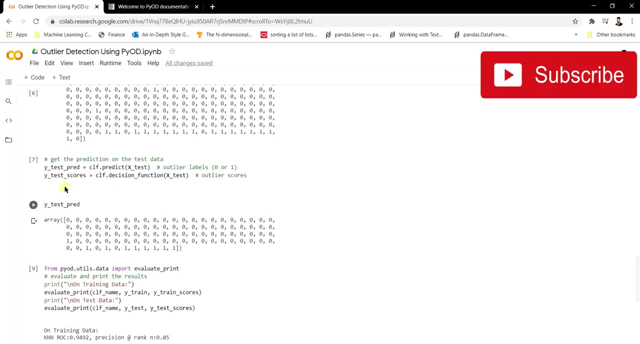 data in it. so we are using this visualization function available from uh piod. so in this, in this visualize function, we are passing this classifier name and x train, y train, x test, y test, and then this y underscore train pad which comes from uh, which is from which comes from this clf method, uh called levels. 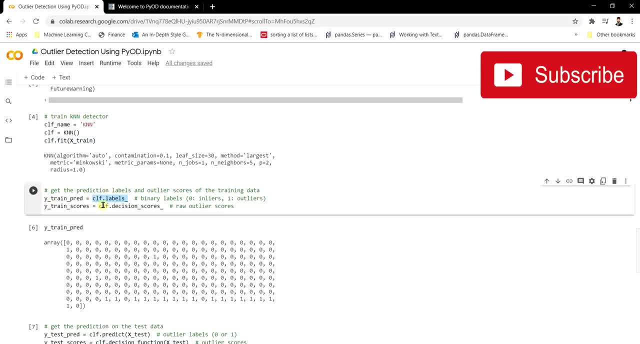 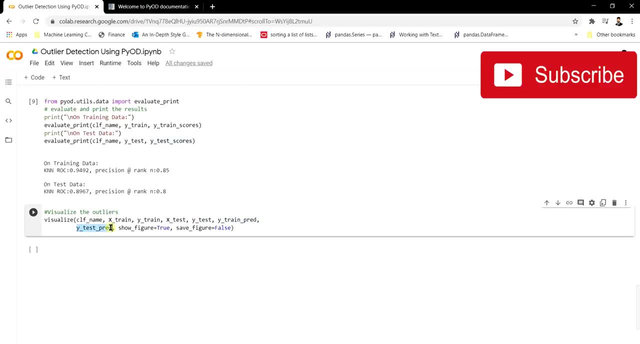 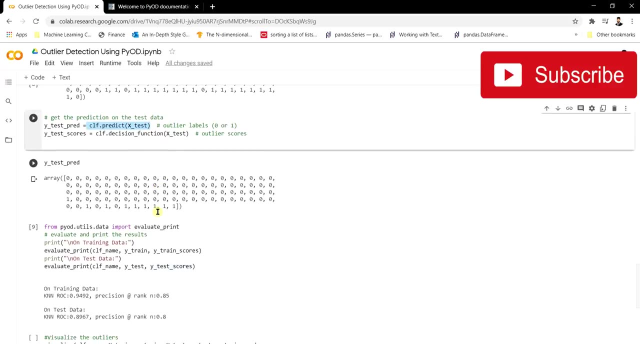 underscore method and it has been stored over here, so it is coming from this, and which has zero and zero, zero and one's value, similarly. so, similarly, we have y underscore test pad, uh, which comes from this function, which is classified dot print. so, whatever, the printed results are coming from uh, from the test data. so it is, it is. 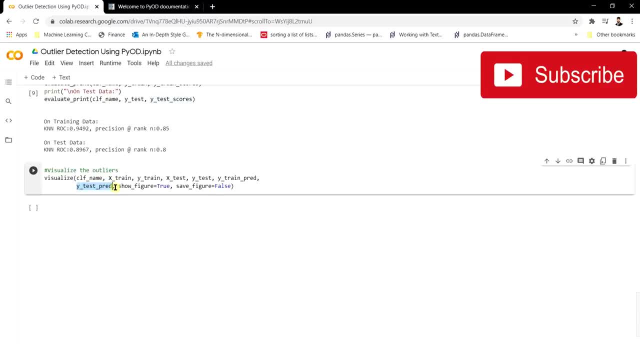 it has been stored in here in this y underscore test spread and which consists of 0 as one, zero and one and similarly: uh, we are, we are, we are passing this uh show underscore figure as true and we're not saving the functions, we are not saving this image, so we are saying that save and 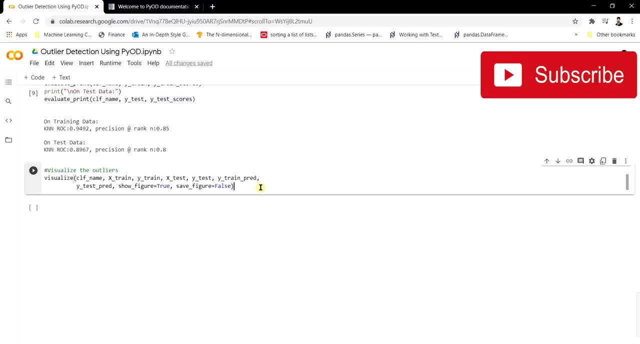 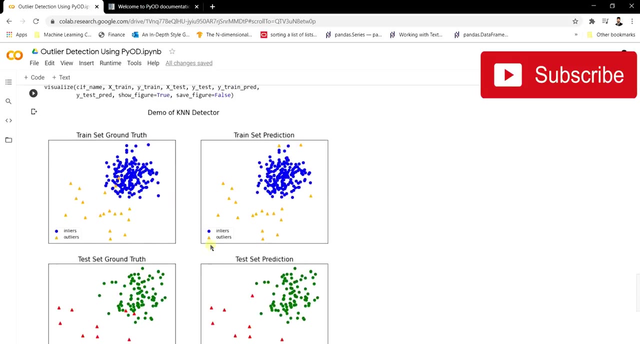 figure is equal to false. so, uh, to get the better understanding, let's run this code and let's see how this, our cloud algorithm, is working. so let's run it. so, as you can see, this is a better visualization over here you can understand with. so these are. 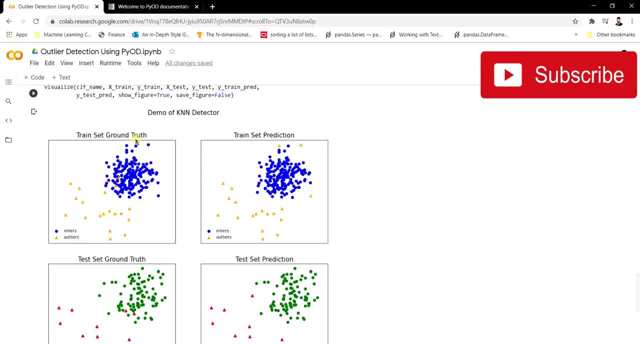 the train set uh, which is ground truth. so it is an actual uh in layers. so these blue points are in layers and these yellow points are outliers in actual uh. that means these are ground truth labels and when these models are being trained on this canon model. so the predicted, the predicted. 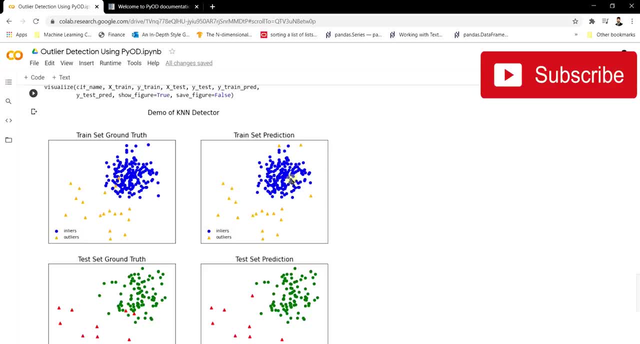 train data set, is it? it's? it is looking like this. so it has printed on the test data like so: these are the inliers and these are the outliers, so you can see few of the points which were actually true over here. it is printed as an outliers and few of the points which are. 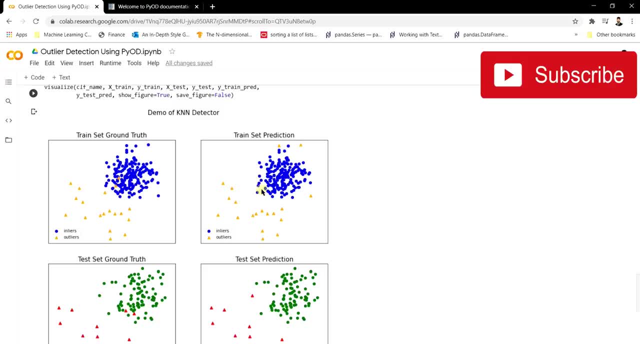 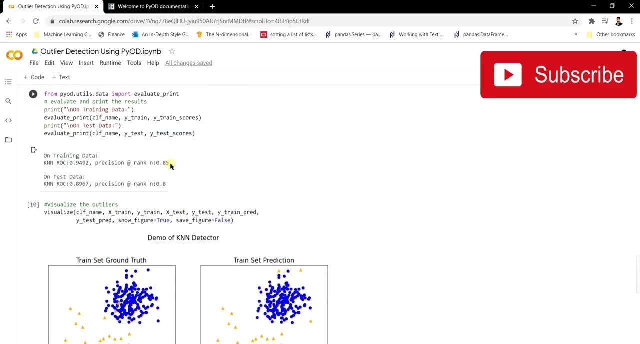 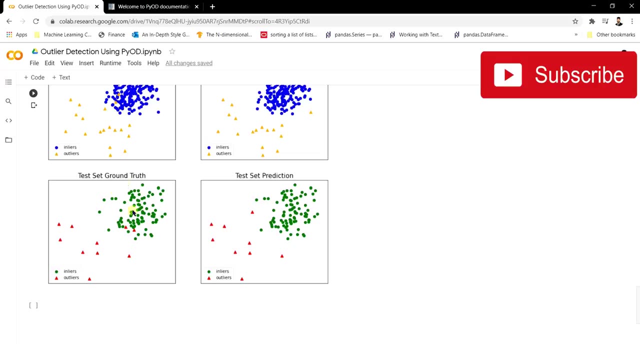 uh, outliers over here as an true label, but it has been classified as an inliers over here while doing the prediction. so that's why our accuracy went down over here, while in terms of precision it's it's 85 percent. similarly, if you see the test test data, so here you have ground truth test data. 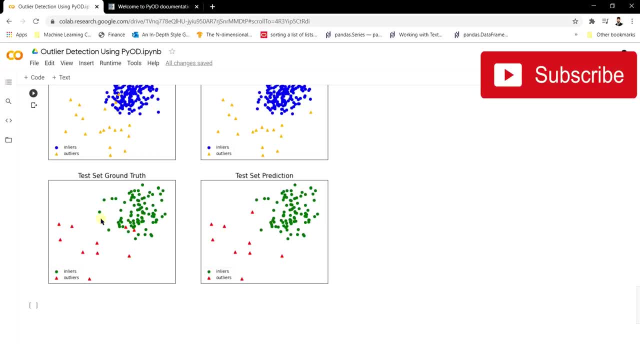 these green dots are inlier points and red are outlier points, but when this model ran into this train, data set, so the prediction performed on this test data are like this. so it has. it has some, some, some points which were outliers over here, but now it has been classified as an inliers and here 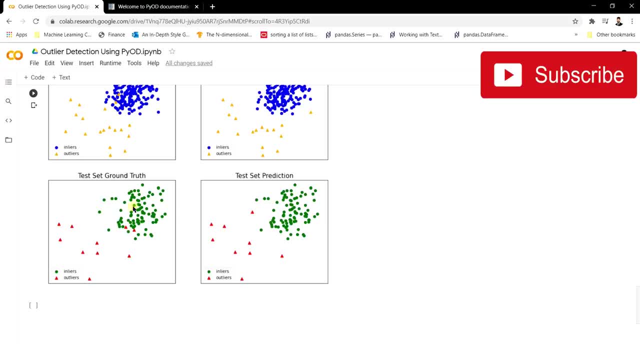 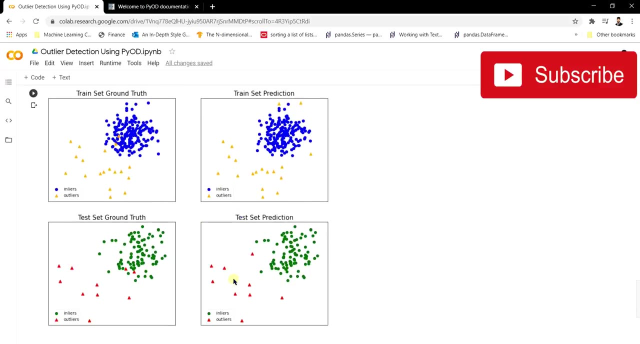 are the few points which were classified as an inliers in in the true, true, true label, as in true label, but it has been classified as an outliers while prediction. so because of these regions, the accuracy went down to 80 percent. so this is, this is the reason why this is happening. we can build a robust model by by. 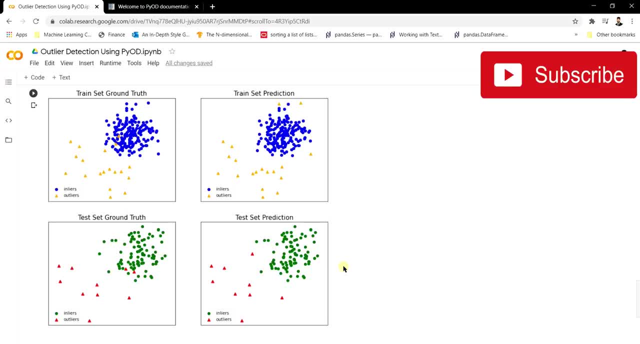 using this PIOD as well by using combining different kind of models as well as using neural network models. so this is how outlier detection is done and hope this version is helpful to understand the proper way of implementation of PIOD. so hope you all enjoyed this video. see you next time. thank you, bye, bye.